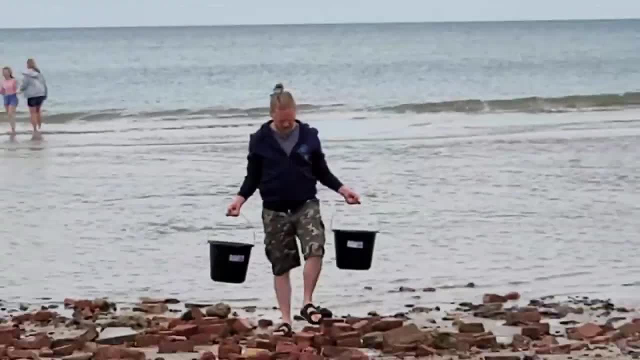 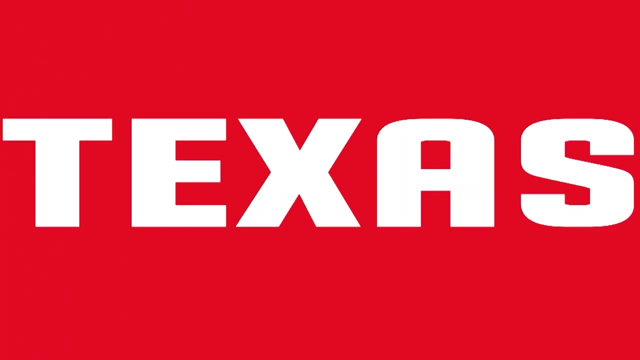 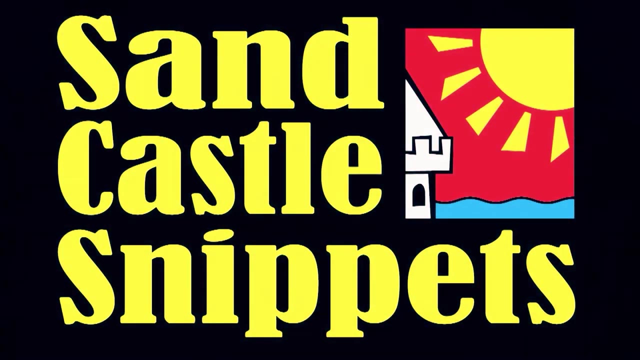 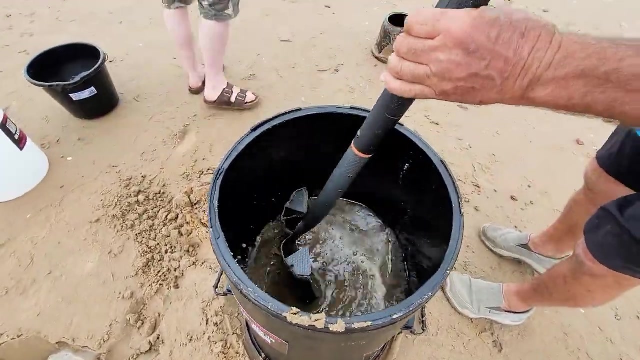 Ah, Sensei, Wax on wax off. Went on wax off. Walter, can you put the water in like that? A bit of a chop. But the one thing is people spend ages jumping up and down, chopping, doing all this other absolute nonsense. 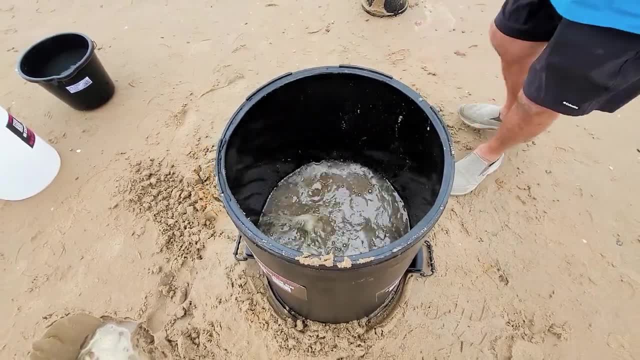 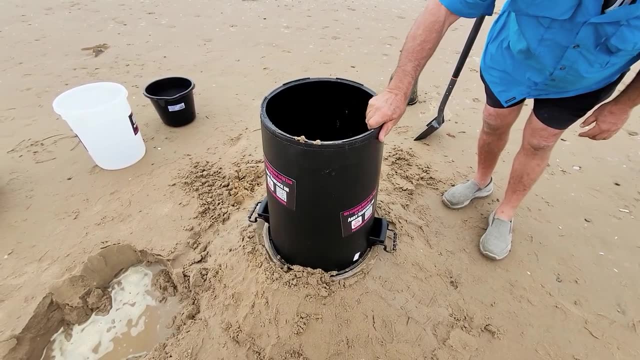 You just chop it up lightly like this, stir it around and then, if you're really sensible, you do this. Look at the bottom. Oh yeah, It has to be a liquid. Don't even think about it, dog. Hello. 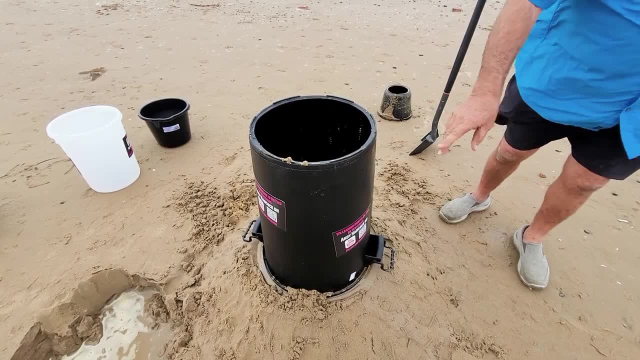 And it has to be a liquid. so if you mix it like that and it comes out as a molten level, you know it's perfectly mixed. If it's wet at the top, wet at the bottom, done, Mmm Boom. 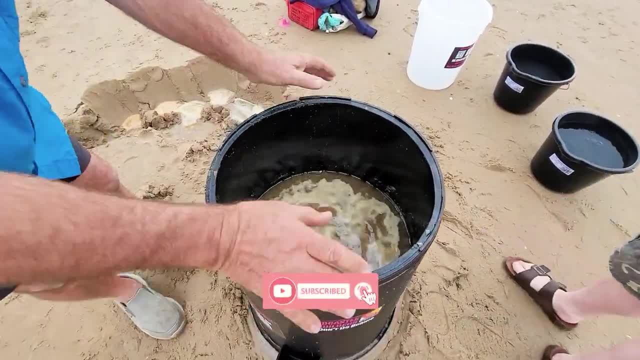 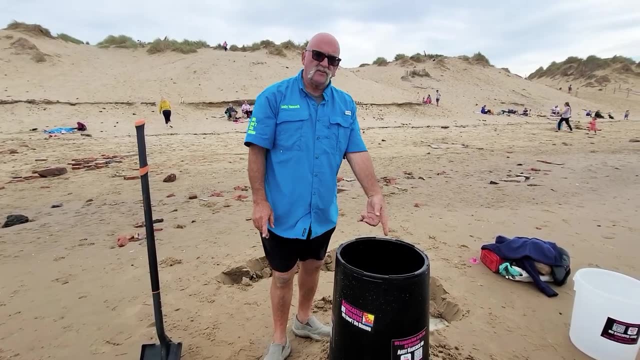 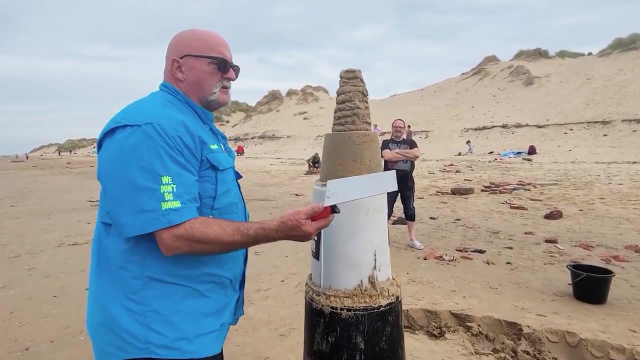 OK, we're going to let this drain a minute because the sand has to settle and lock itself together. Yes, because there are four states of sand: Molten, pendular, funicular and capillary Ready. Oh, by the way, remember that noise. 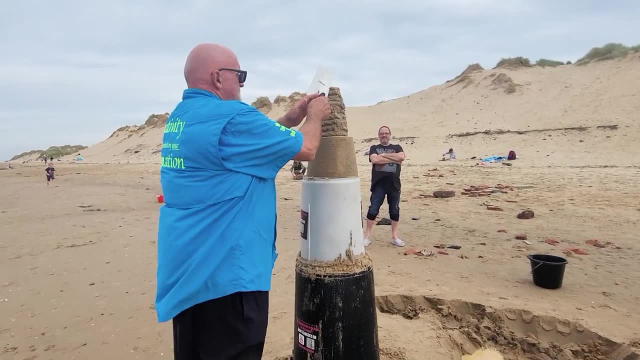 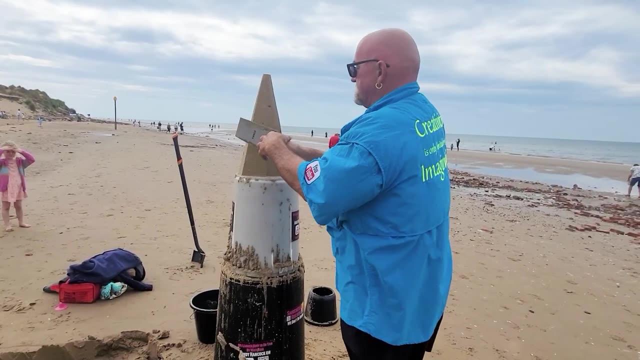 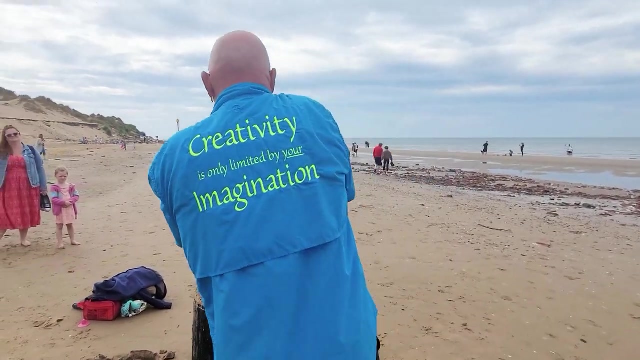 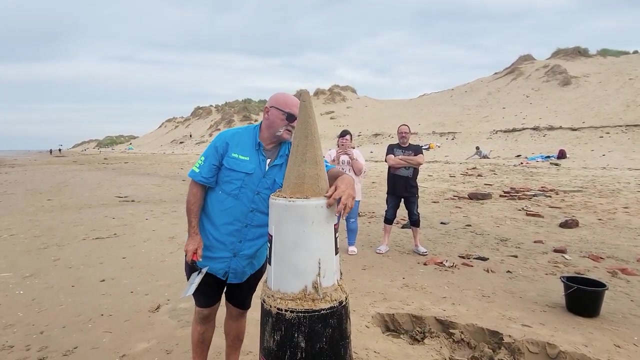 It's going to fall over, is it? I don't think so Ready. The reason we're using this different tool like this is because you get a nice flat edge Occasionally, And then this is where you have to hope to hell your lube works, because if it doesn't, you're in big trouble. 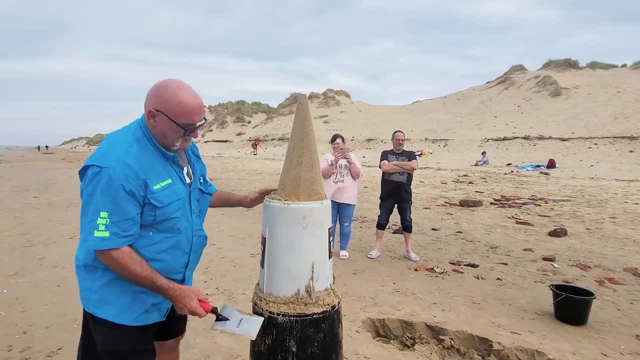 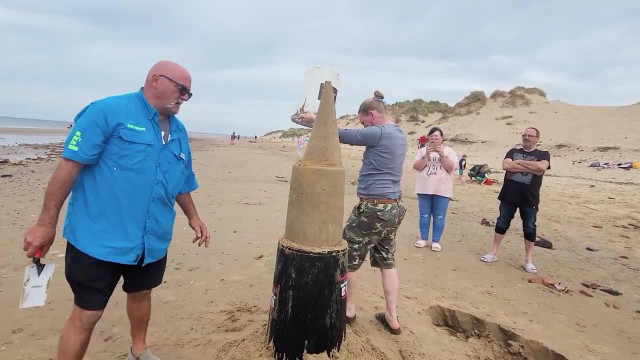 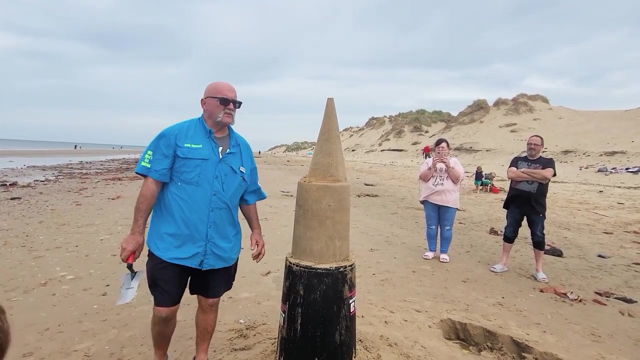 You have to spray the inside of the buckets. Whoa Ta dah, Ta-da. Ooh on me, edge On your edge, Ta-da, You wanna try that noise again? Ta-da, Ta-da, Ta-da, Ta-da. 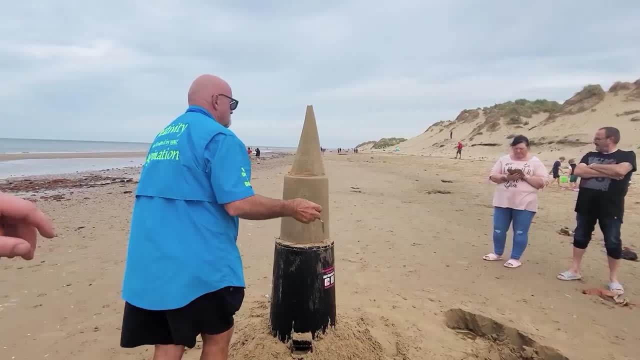 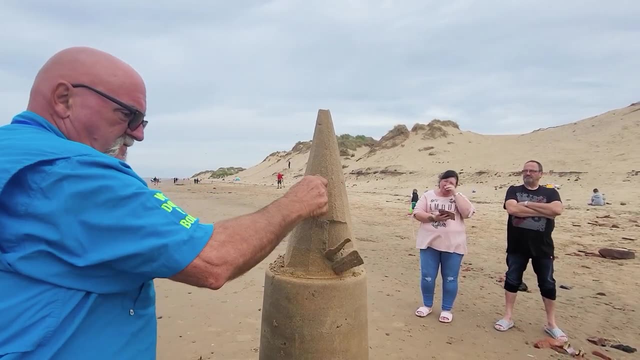 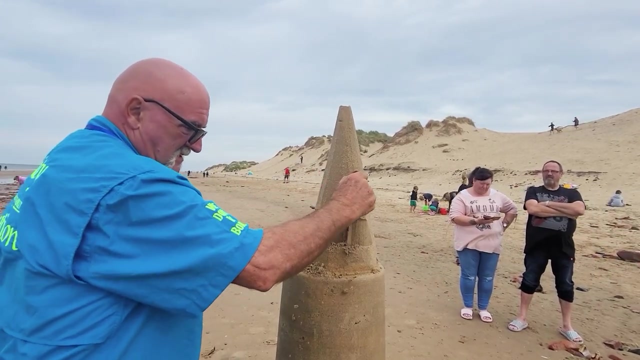 Oh yay, Oh yay, A little different. And then, if you want to tower, you put it like this: because it's got a bump in it and you do this, and that way you can make a perfect tower every time. now the other thing. 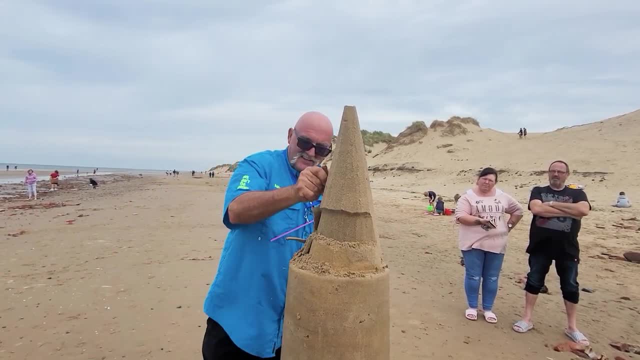 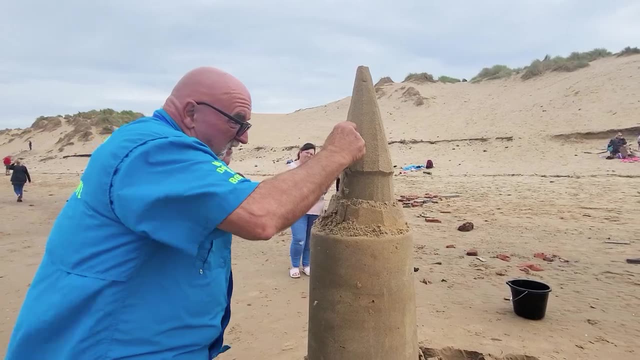 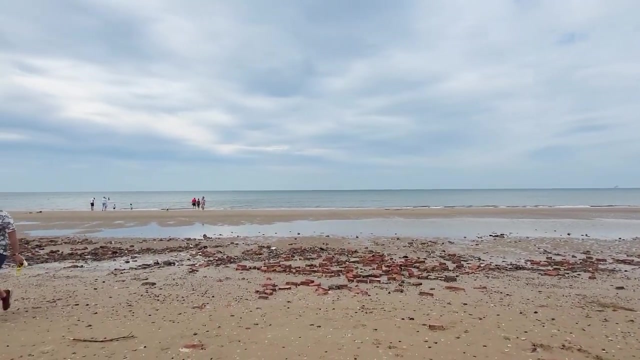 ladies and gentlemen, is how do we tell that this line is straight? we've got on a beach with no level. there's no water left. how can we get the top of our tower straight? what do you call that line between the sky and the sea? young lady, 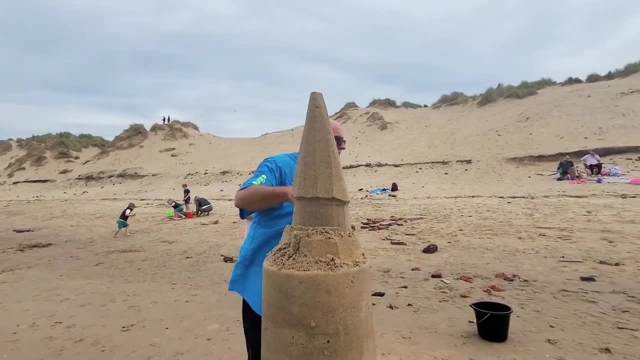 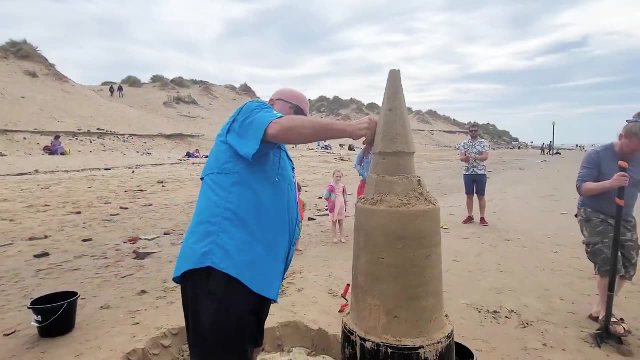 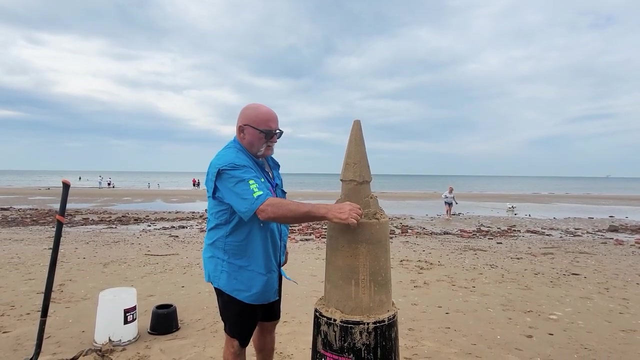 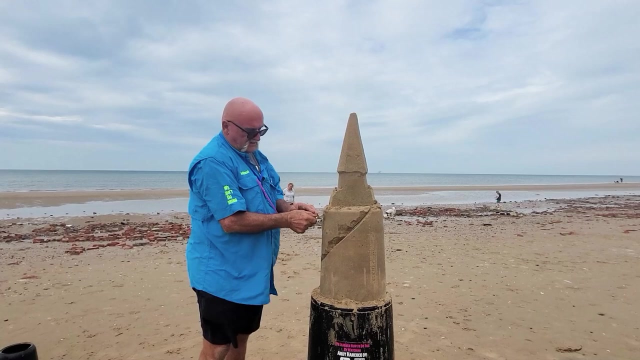 why do you like your top? I know it's a miracle. like I said, this is the real science division, not the rocket science. do we make stairs? I don't know how do we make this? we start with a ramp. you cut the diagonal line right into it- butter. 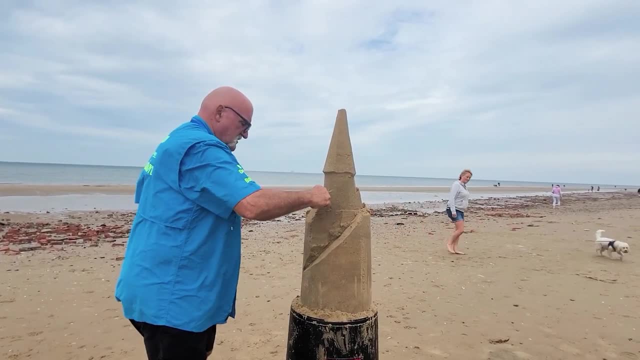 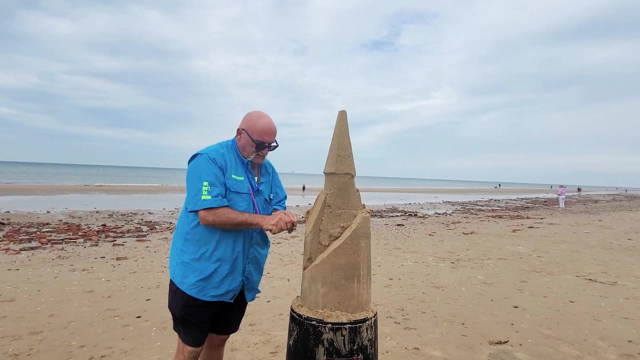 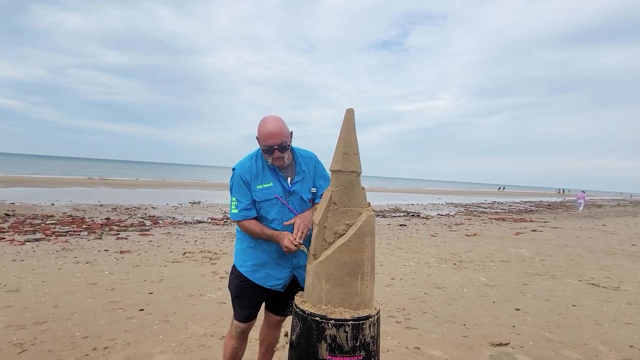 I know it's a miracle. we want a nice long castle building here, so we're gonna chop that line down there and chop that line down there, chop this line here, and then we're gonna chop in like this: so we got somewhere for our stairs to go. 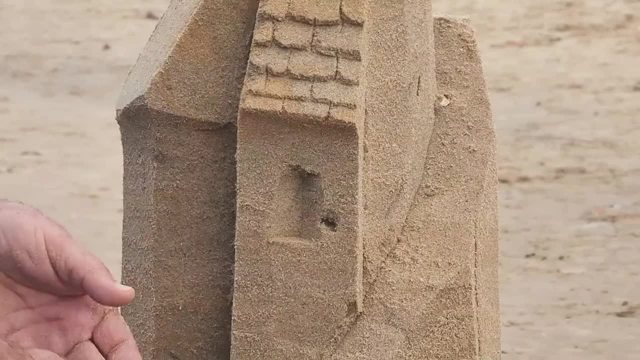 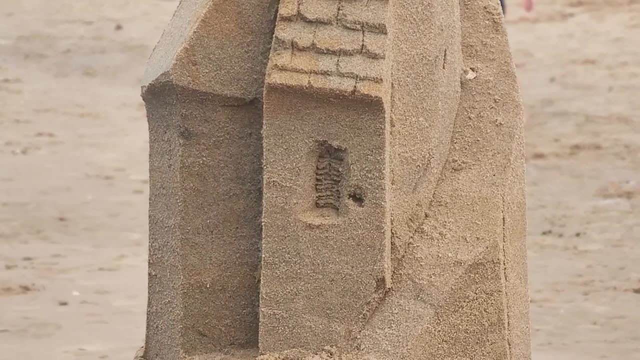 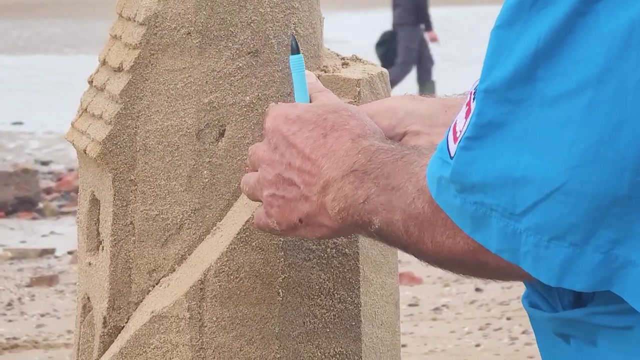 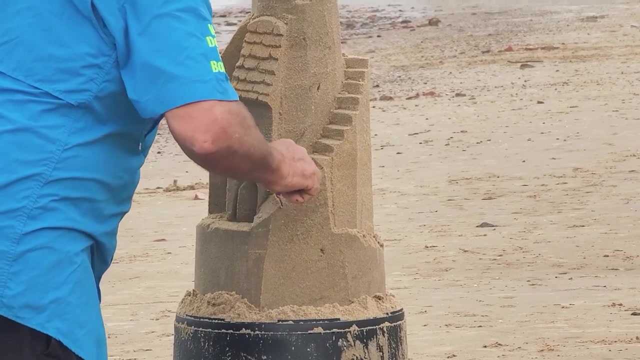 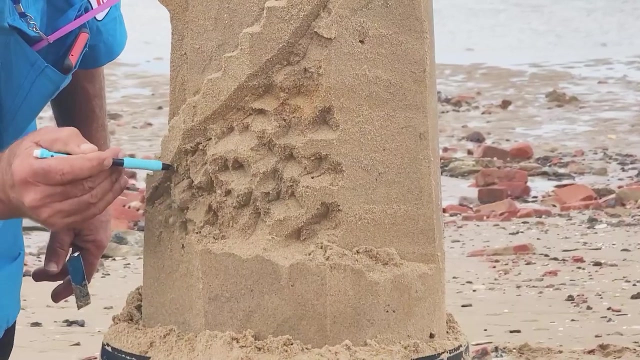 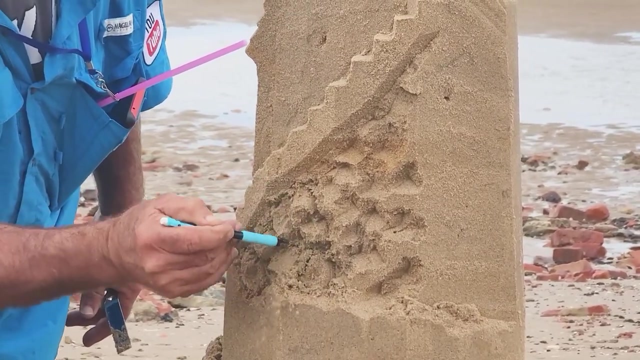 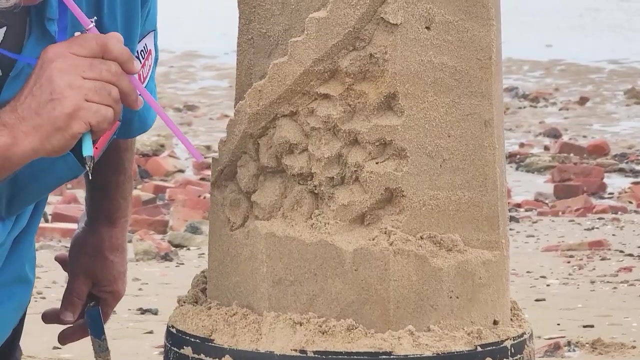 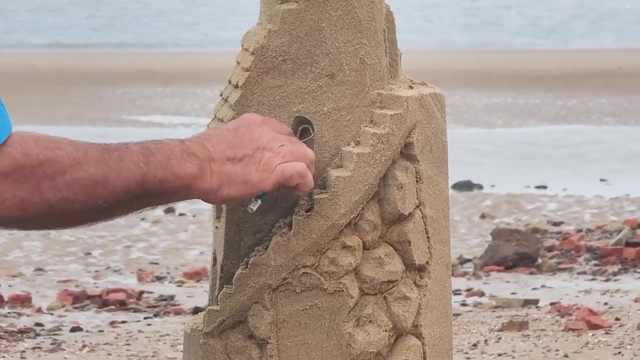 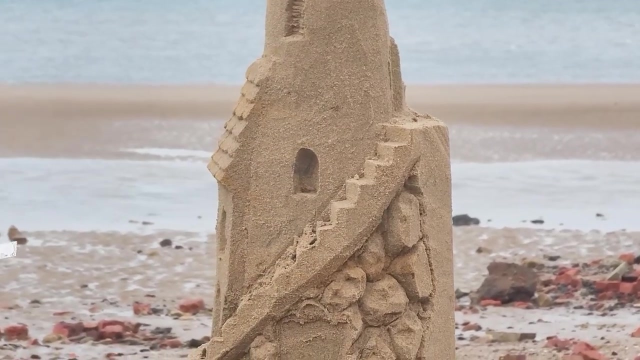 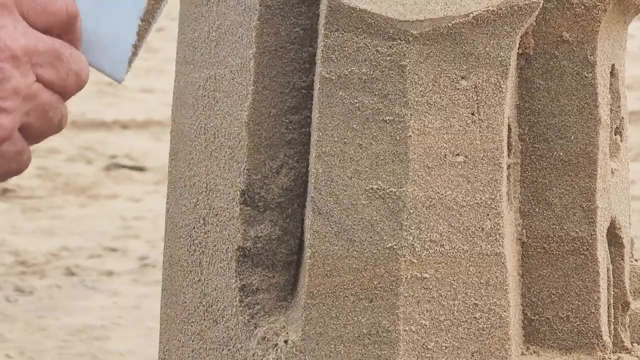 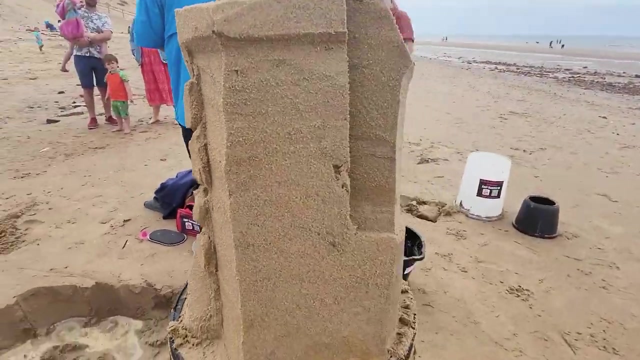 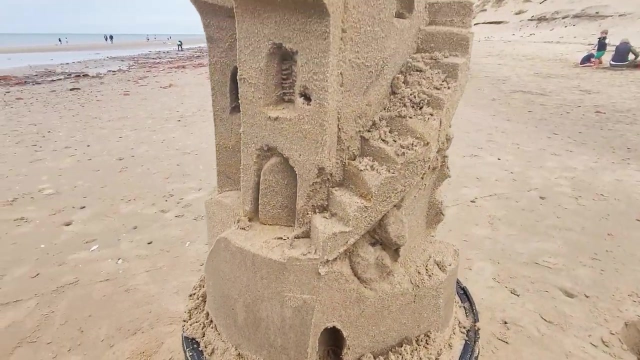 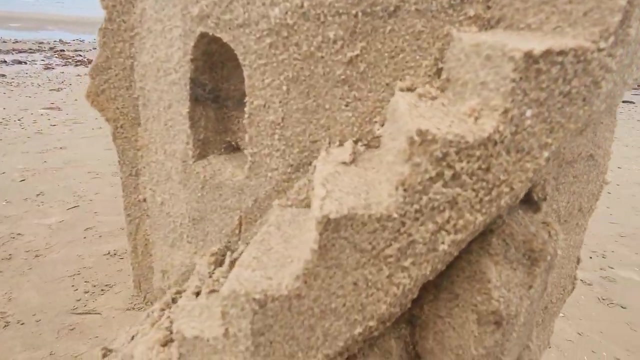 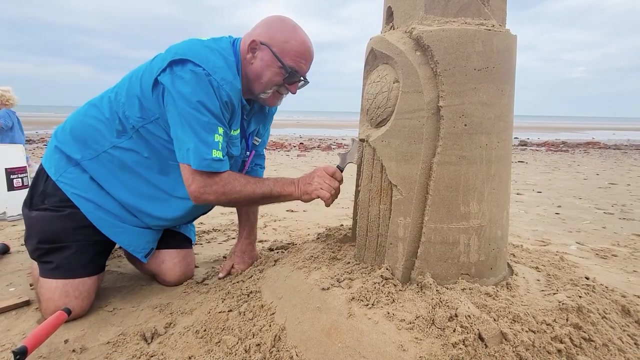 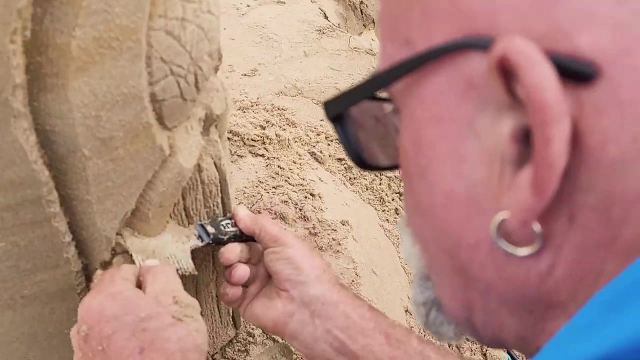 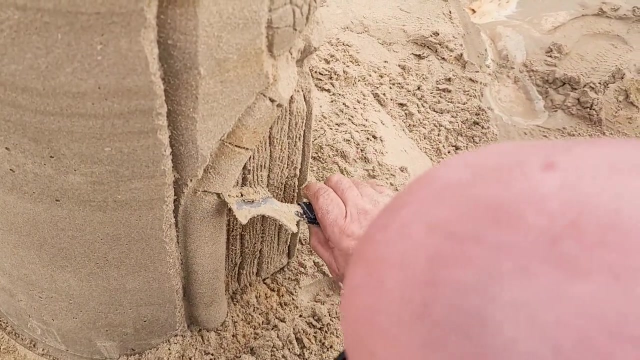 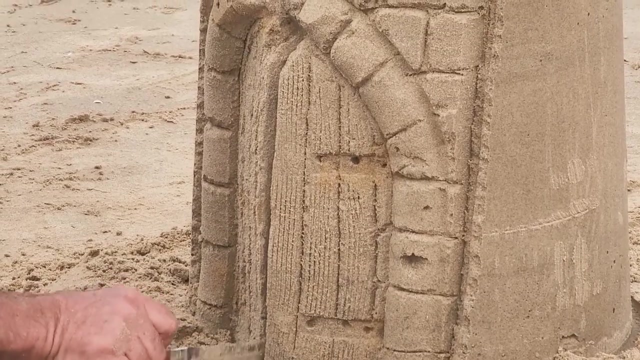 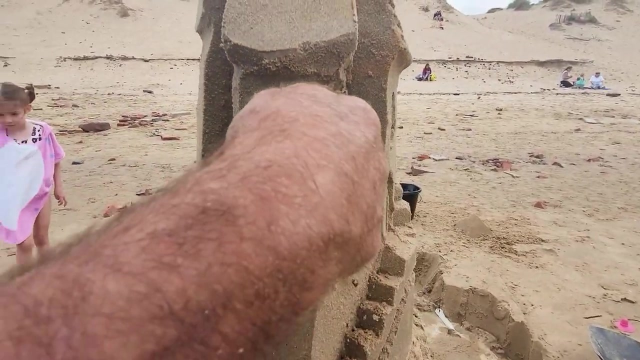 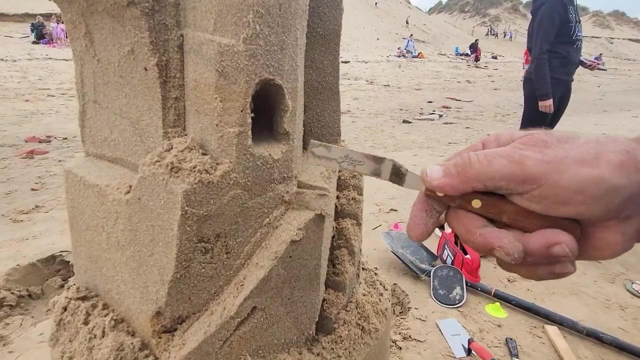 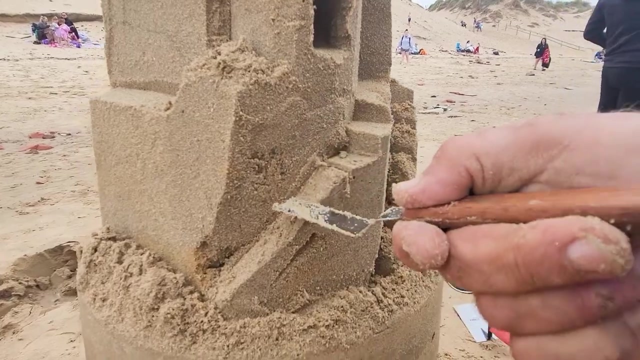 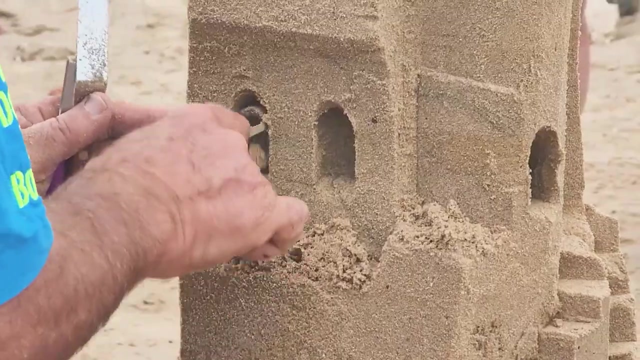 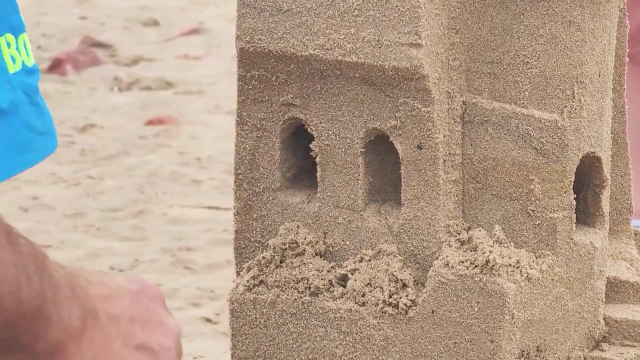 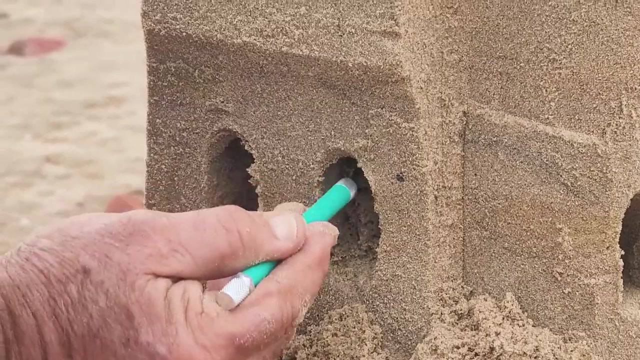 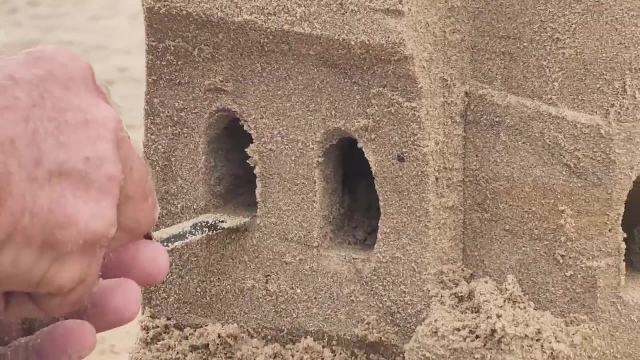 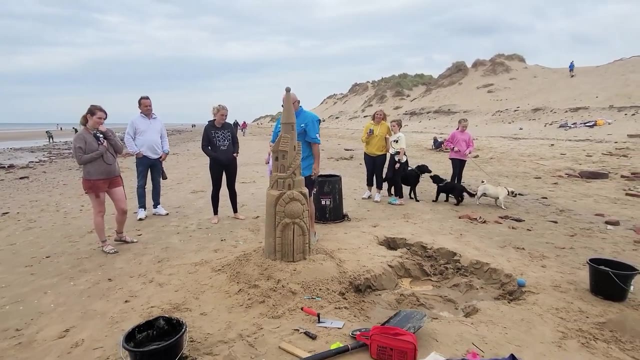 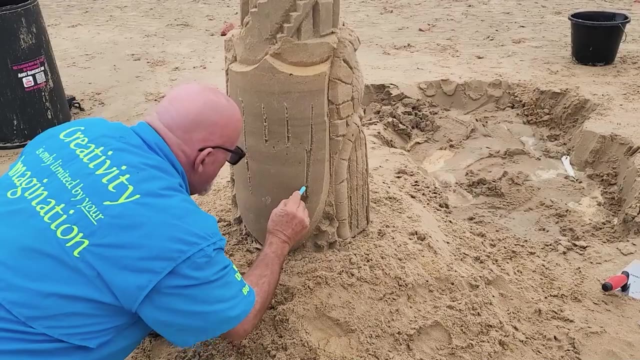 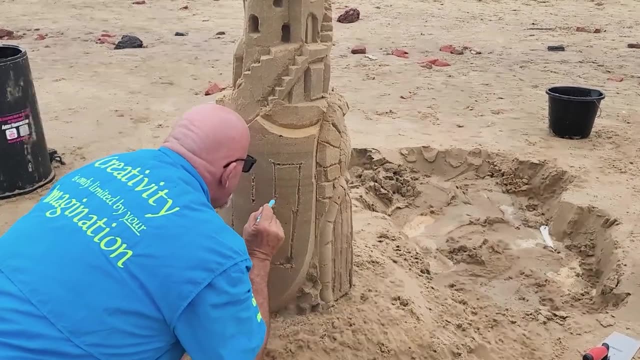 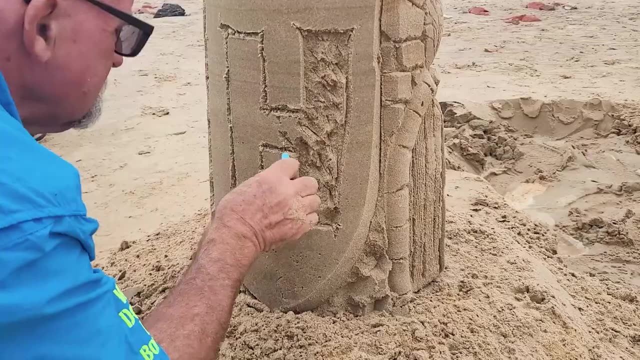 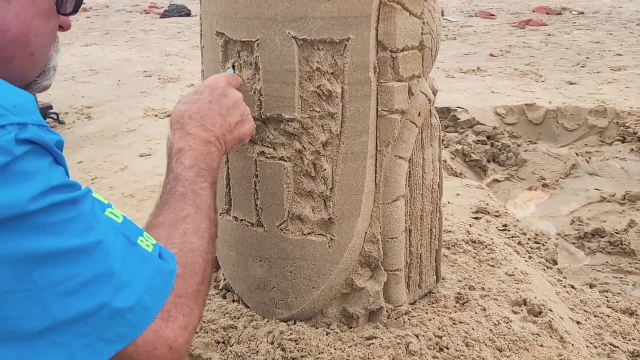 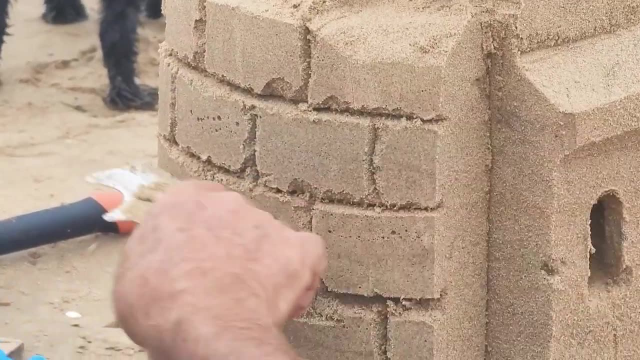 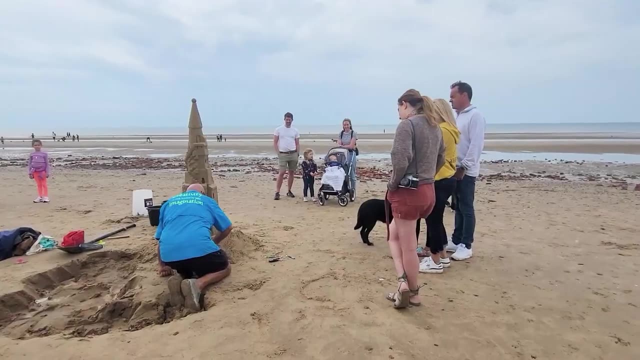 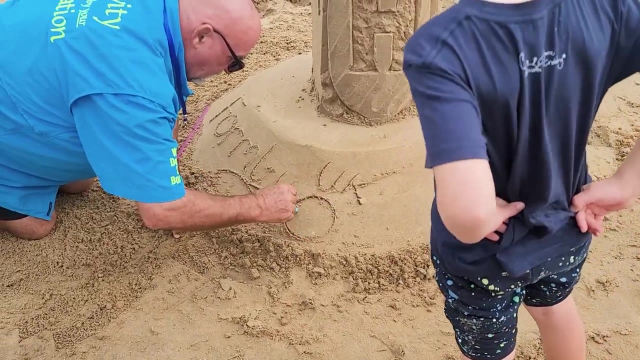 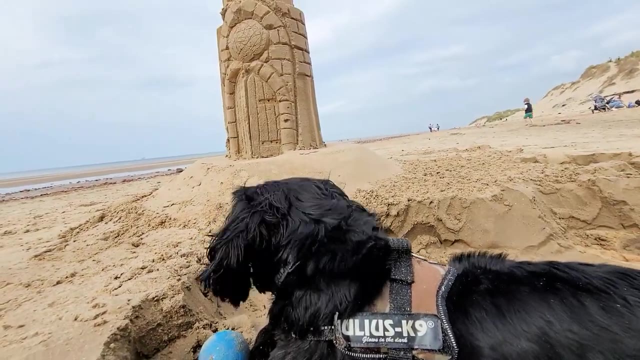 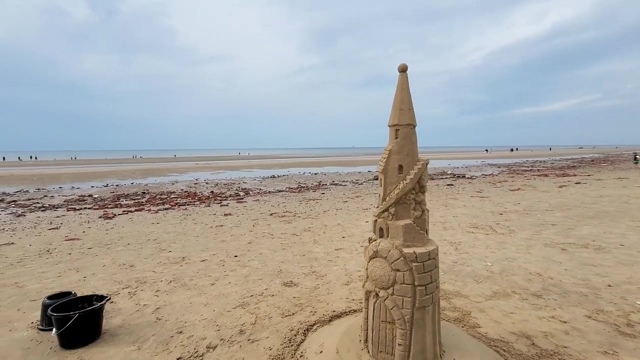 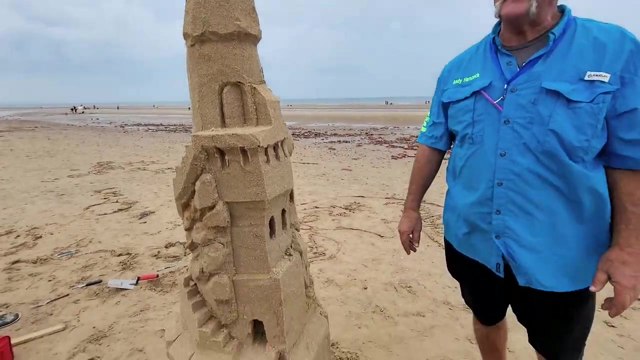 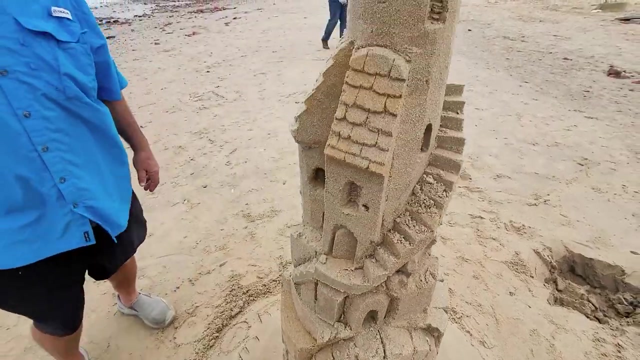 because this will be our door, you, you. so, hey, welcome back here. we go there, it is. we've. we proved that Formby in England is the place to build a sandcastle. look at this, this is a. well, it's at least as tall as me, so that's 5'8 and it's got all the details on we.